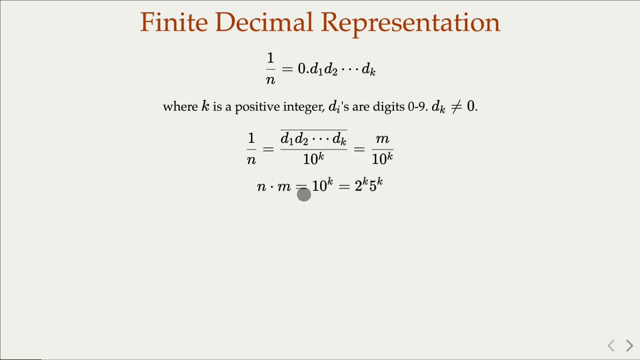 you know that n and m multiplication would get 10 raised to kth power. so which means n contains only factor 2 and 5. okay, so cannot contain any other prime factor other than 2 and 5. that's the proof. now how about for the fraction? 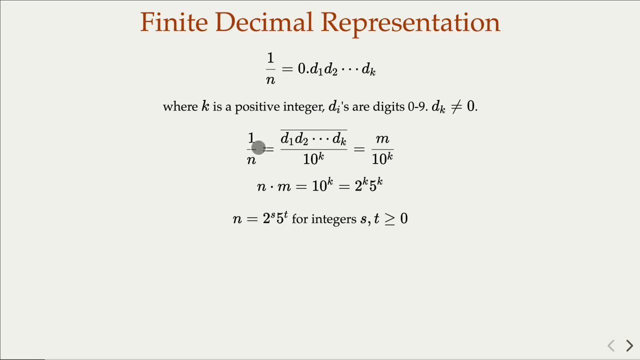 that the numerator is not 1, do we make the same conclusion? the answer is yes, so the same argument here. we assume m is a smaller and m and n are co-prime. okay, so it's a finite digit here. by the prior argument, we have this: 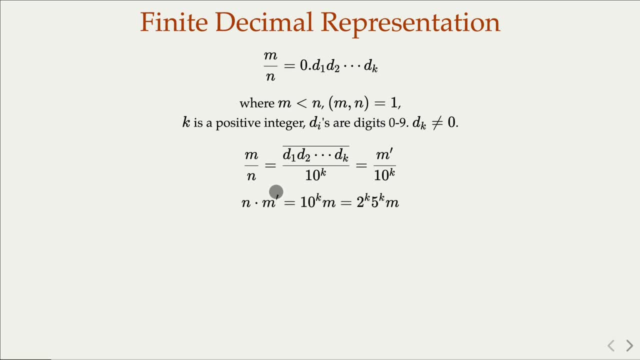 okay, so we have a finite digit here by the prior argument. we have this. okay, so we have a finite digit here by the prior argument. we have this. okay, so we have a finite digit here by the prior argument. we have this now. this time we're gonna have the product. 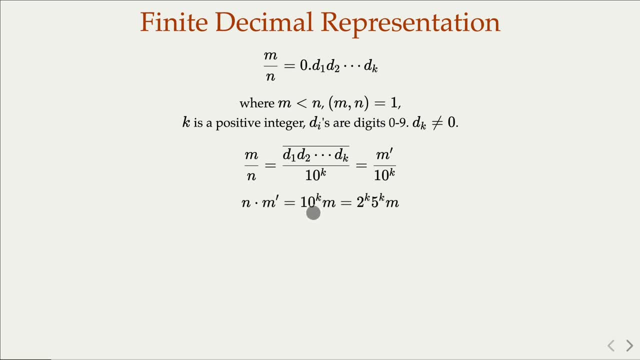 now, this time, we're gonna have the product. now, this time, we're gonna have the product equal 10th power times M, however, since equal 10th power times M. however, since equal 10th power times M. however, since n and M are relative prime, we're going to. 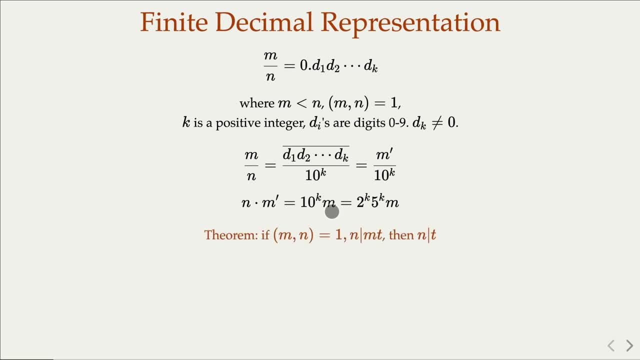 n and M are relative prime. we're going to n and M are relative prime. we're going to use one number theory basic theorem. use one number theory basic theorem. use one number theory basic theorem, that is, if two number are co-prime and n. that is, if two number are co-prime and n. 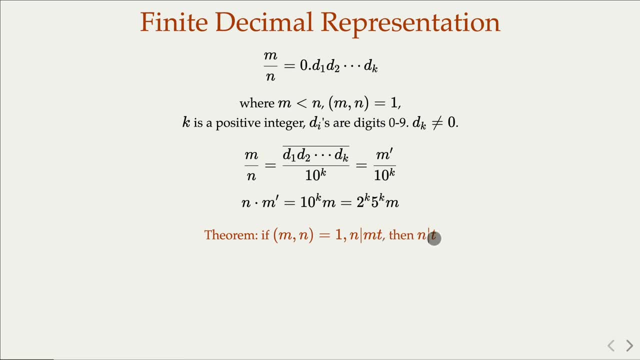 that is, if two number are co-prime and n divides m times T. in this case, n has to divides m times T. in this case, n has to divides m times T. in this case, n has to device T. now apply T to 10th kth power. 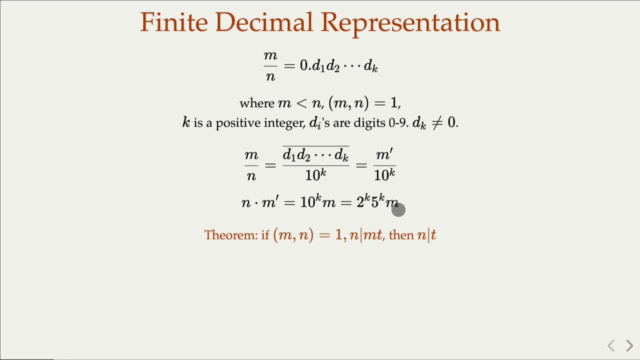 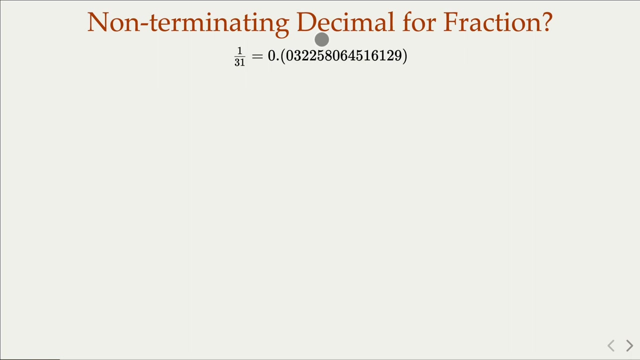 here. in our case we say that N and M are relative to prime. so that means N has to divide 10 to the case power. yeah, So from there we conclude that N cannot contain any other prime factors. right, So that's the proof. but what about the non-terminating case? right? So, for example, 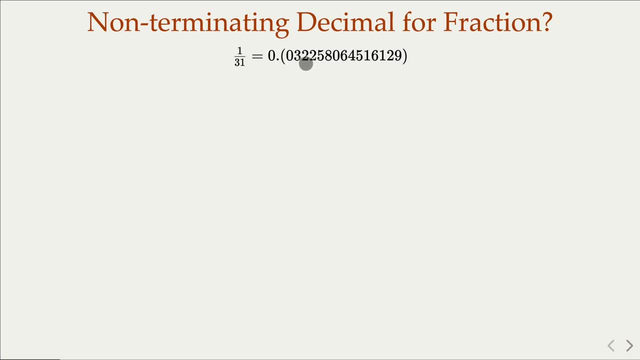 this notation here, meaning the repeating decimal. here, in this pattern it's going to repeat. and there's another example with a shorter period length and 49 is even longer one. okay, This is 42 digits here. Now we're going to look at the period length for the case where